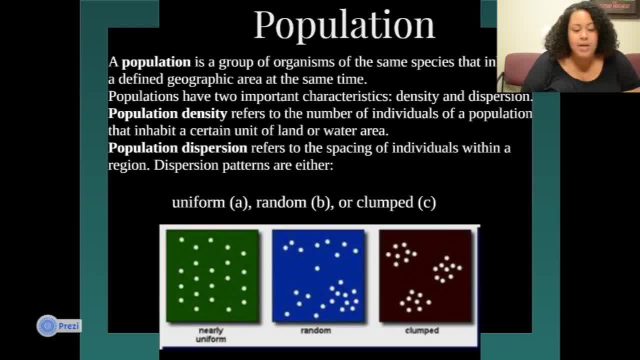 inhabit a defined area. at the same time, Populations have two important characteristics, which are density and dispersion. So population density refers to the number of individuals of a population that inhabit a certain unit of land or water, And population dispersion refers to the spacing of the individuals within a region. Dispersed patterns can either be: 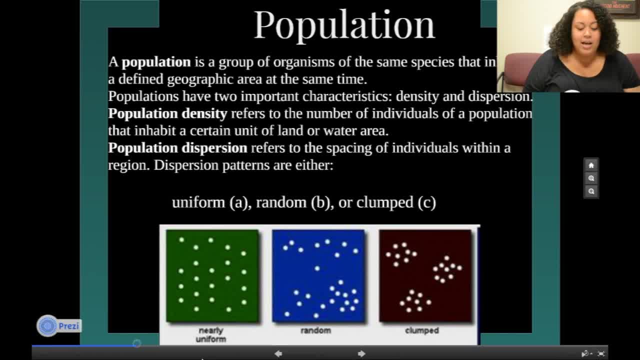 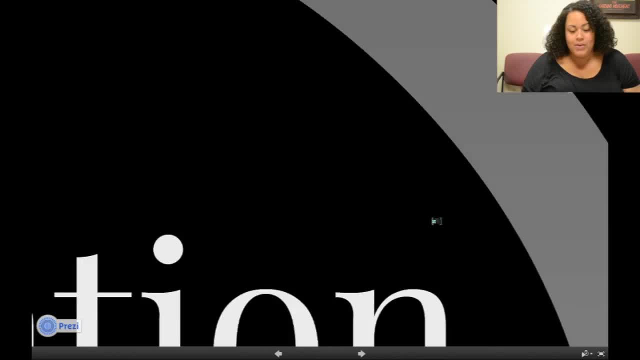 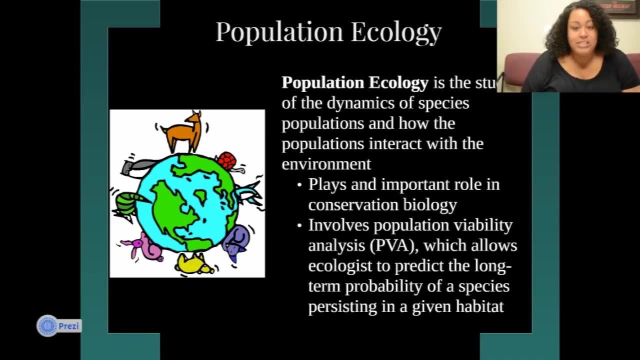 uniform, random or clumped. In this picture it's either uniform like this, random like this, or clumped up like this. Population ecology is the study of the dynamics of species, populations and how the populations interact with the environment. It plays an important role in the conversion, the conservation, 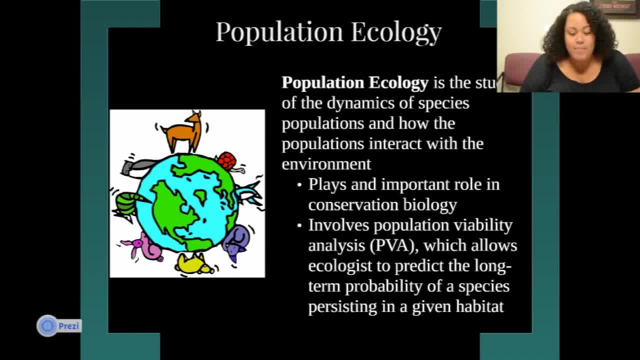 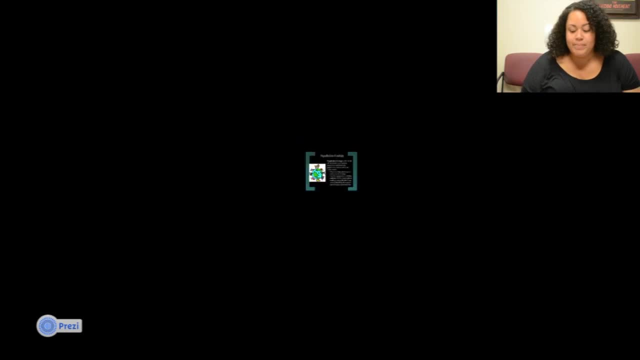 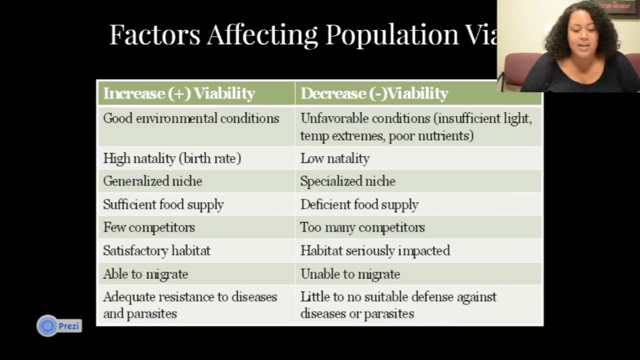 of biology. It involves the populations' vulnerability to the environment. It involves the population's vulnerability analysis, which is PVA, which allows ecologists to predict the long-term probability of a species' persistence in the given habitat. So these are factors that affect the population's viability. So some increases of the viability. 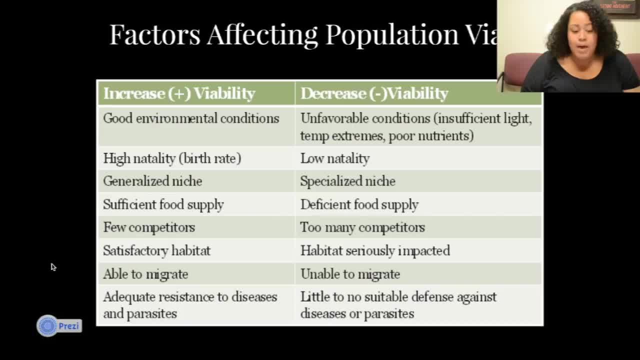 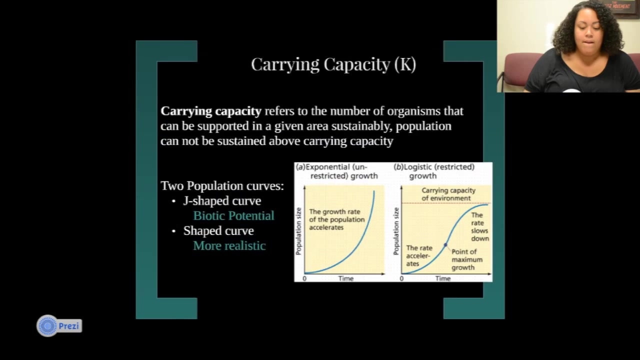 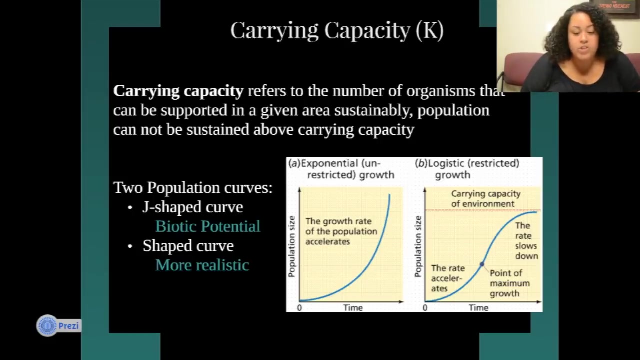 are good environmental conditions, few competitors, sufficient food supplies and the ability to migrate. Some things that decrease the viability are unfavorable conditions: low nationality, specialized niche, deficient food supply and too many competitors. So the carrying capacity, which can also be called K, refers to the number of organisms. 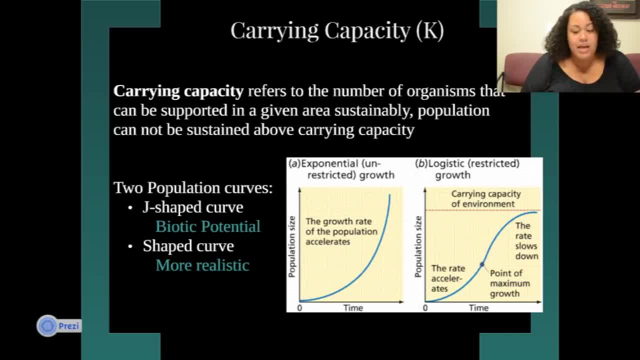 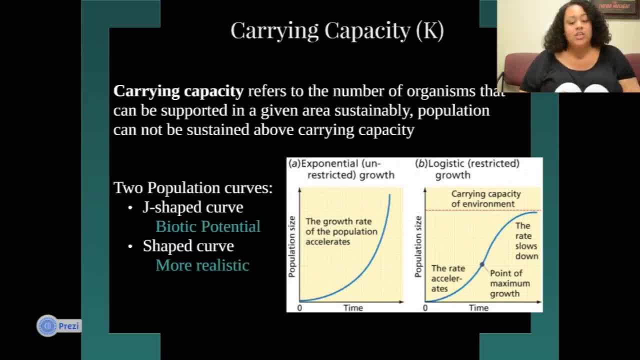 So the two main curves that you need to know are a J-shaped curve, which is the biotic potential, That's exponential growth, That's unrestricted growth, That's how human growth was for a very long time, And the S-shaped curve, which is actually the more realistic. 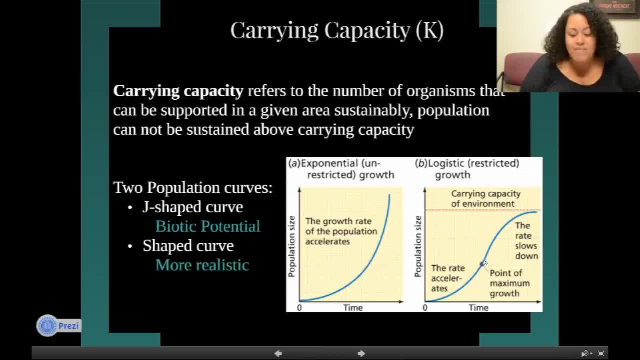 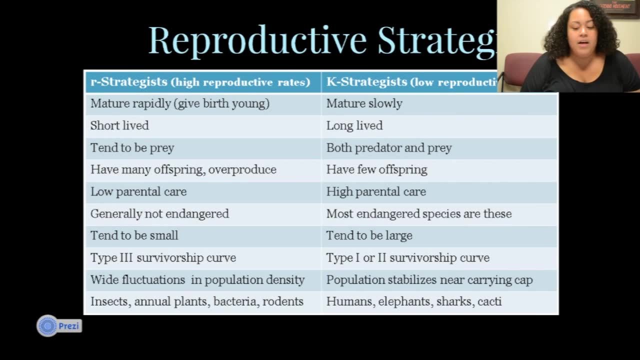 So it starts off as a J-curve until you reach a point of maximum growth And the growth rate slows down As it slowly reaches the carrying capacity. Here's some reproductive strategies, And those strategies are R-strategists, which have high 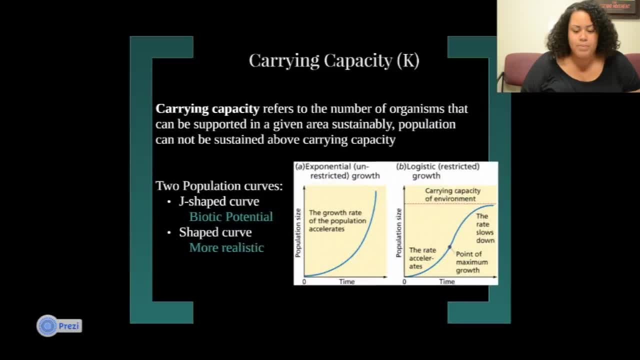 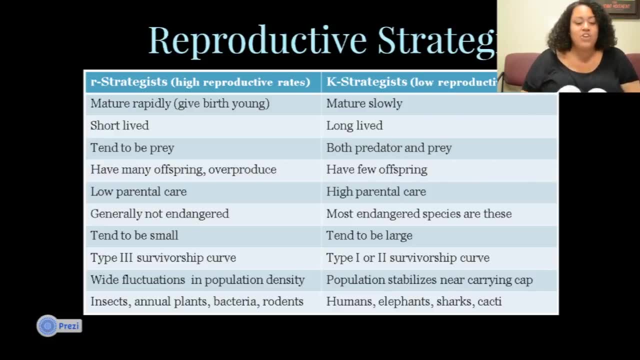 reproductive rates and K-strategists with low reproductive rates. Oh my bad. But here's back to the graph. So, as you can see through the graph, R-strategists- they mature more rapidly And K-strategists mature more slowly. 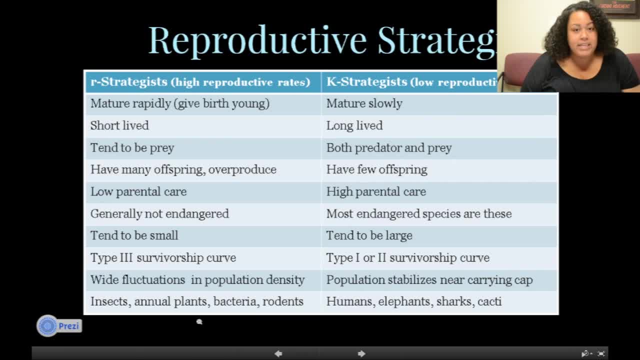 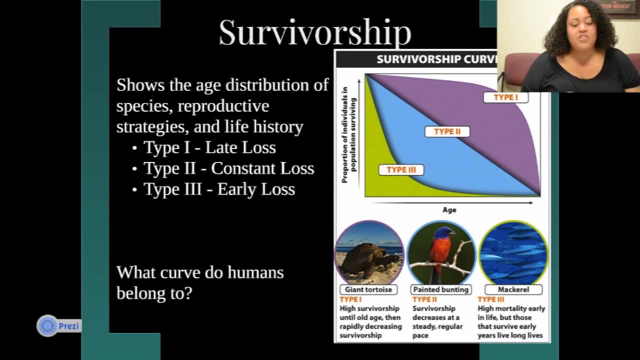 R-strategists are things like insects, animal plants, bacteria, rodents, While K-strategists are usually bigger. animals like humans, elephants, sharks and even cacti are considered K-strategists. So, as you saw, there's a sponsorship curve. Let's talk about that real quick. 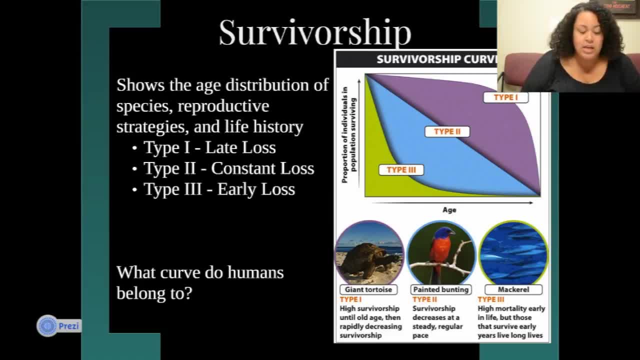 So the sponsorship curve shows the age distribution of a species and reproductive strategies and its life history. So type 1 is a late loss. They're really strong at the beginning and then just come off. Type 2 is a constant loss, which is a straight line all the way down. 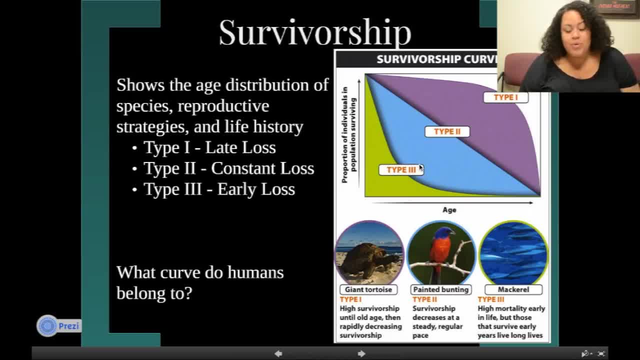 And type 3 is an early loss. So type 3 would be like insects: you lose a lot very early. Type 1 would be like birds: They slowly die off. Type 1 would be like giant tortoise. 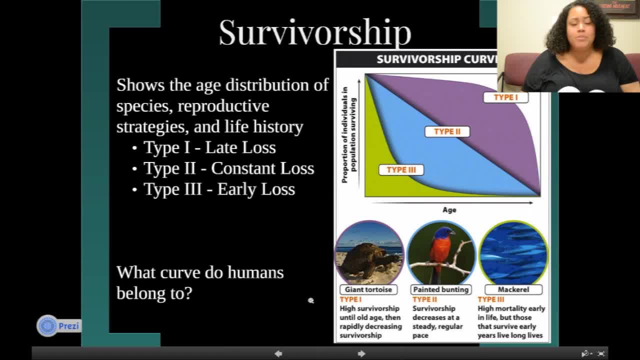 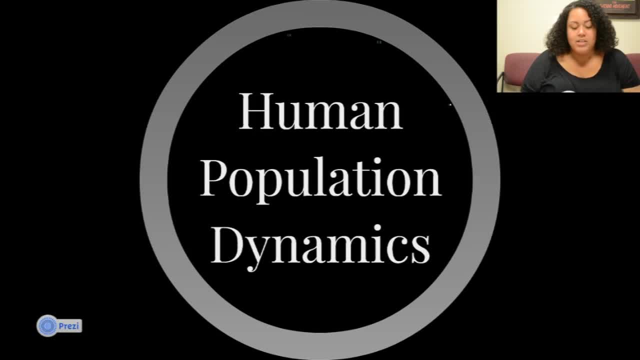 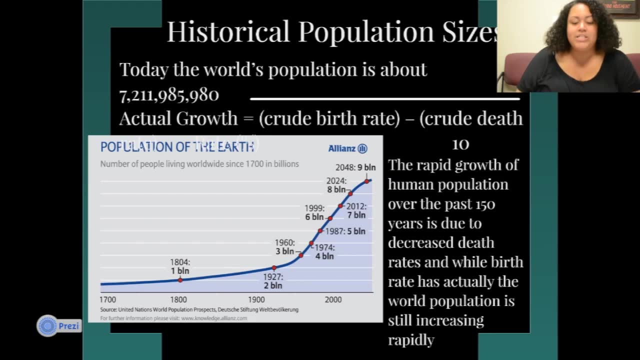 old and all of a sudden they die of old age. So what curve do you think humans belong to? I'll give you a hint: we're a lot like a tortoise. So human population dynamics. There's a next one up. So historical population size. Today's world population is about 7 billion. my bad. 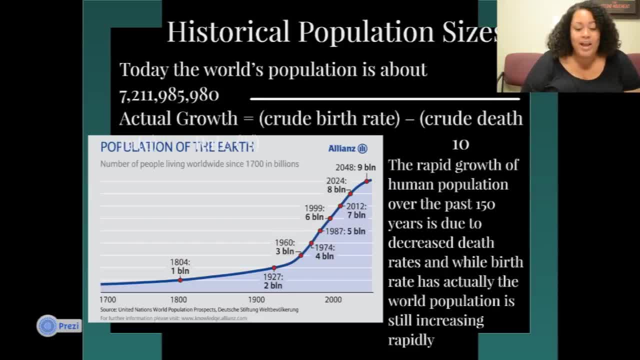 200 million and it's forever growing. The animal growth rate comes from crude birth minus crude death. it should be over 10.. The graph got kind of messed up here. The population of earth, as you can see, is showing a rapid growth. Where we're at right now, we hit 7. 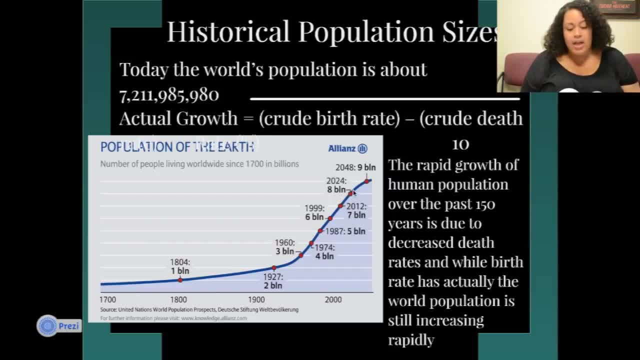 billion in 2012 and we're predicted to start growing again in the next year or so. We're going to start slowing down our growth. The rapid growth of the human population over the past few years is really due to decreased death rates, While birth rates have actually. 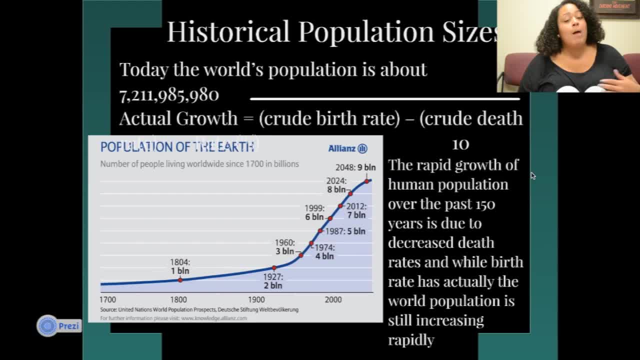 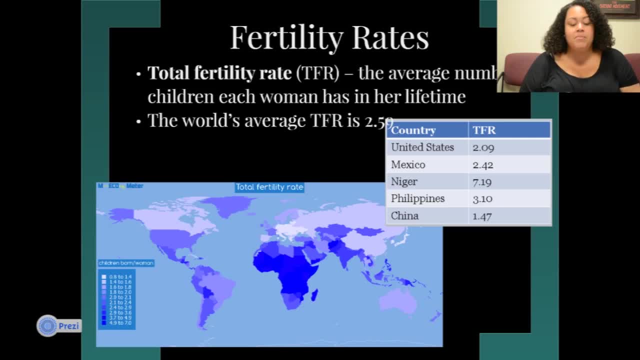 dropped in the world population. the earth's population is still rapidly growing. Fraternity rates are something that really has to do with this. Total fraternity rate, or TFR, is the average number of children each woman has in her lifetime. The world's average. 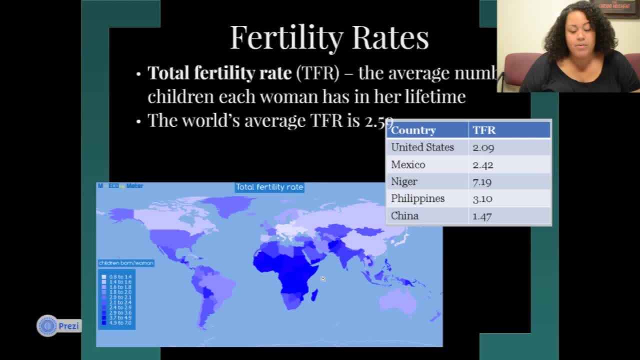 TFR is actually 2.59 right now. Every country differs, though: The United States is 2.09,, in China it's 1.47,, in the Philippines it's 3.1, and in Niger, which has the largest TFR. 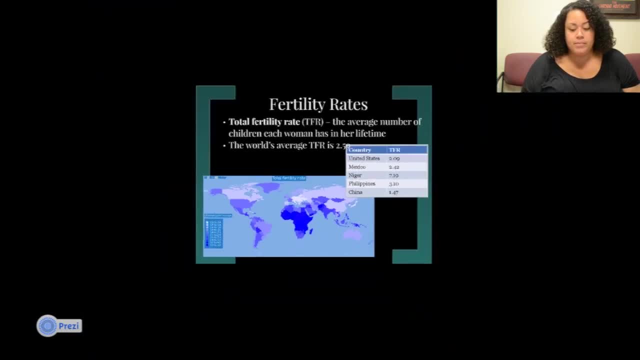 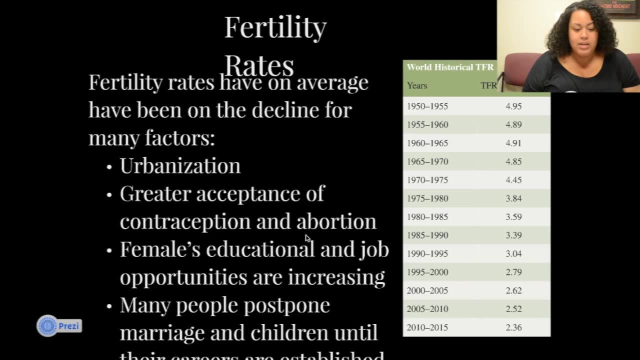 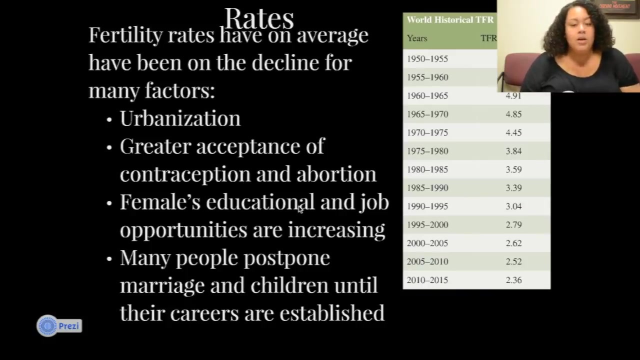 in the world. right now it's 7.19.. Fraternity rates- The world's average TFR, has been on the decline because of many factors: Urbanization, the greater acceptance of condom use and abortion. females educational and job opportunities are. 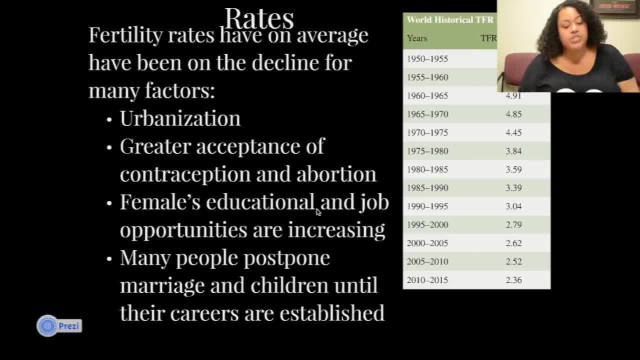 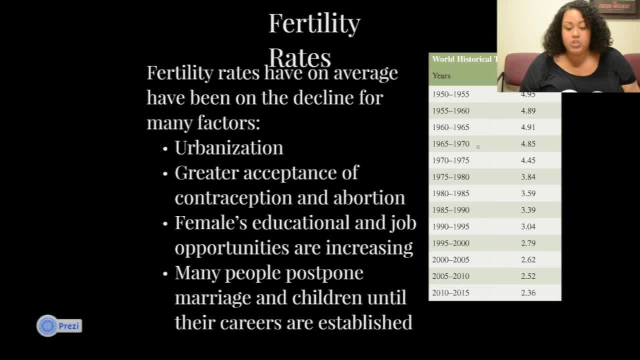 increasing and many people postpone marriage and children until later in life when their careers are established. Here. this shows the world's historical TFR As you can see: the 50s it was almost 5 years, all the way almost to 5, while today it's been slowly decreasing all the way to 2.3. 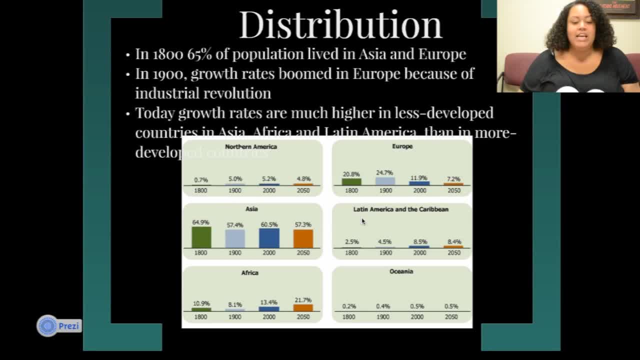 distribution. in 1865 the population lived in Asia and Europe. by 1900 the growth rates boomed in Europe because of industrial revolutions. today's growth rates are actually much higher in less developed countries in Asia, Africa and Latin America, more than the developed, more than more developed countries. this 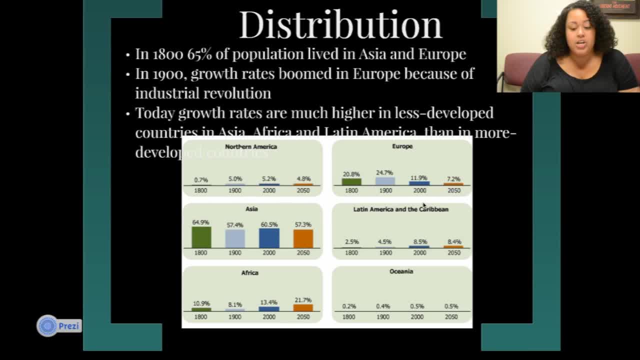 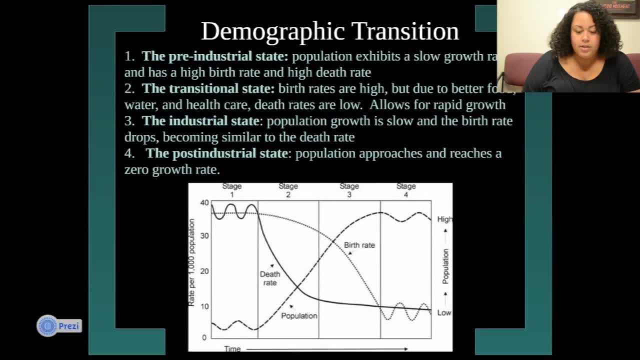 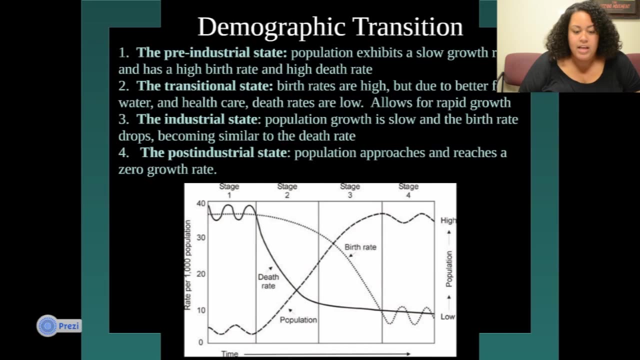 graph right here shows the distribution of the world's population over time, from all the way to the day to what's expected in the future. demographic transition is how we know how countries and stuff like change the growth rate. so you have: the pre-industrial state is slow, death rate is high, birth rate is high, traditional. 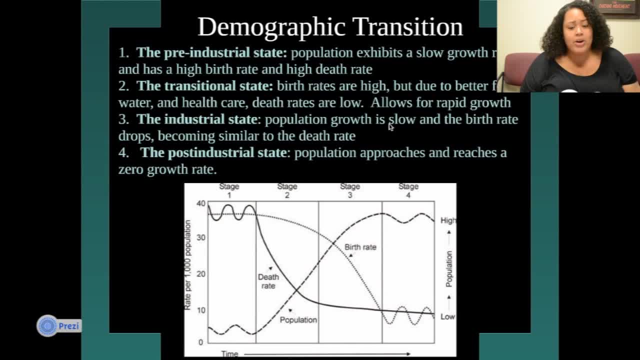 state, the birth rates are still high, but due to better food, water and healthcare, death rates are low, which allows for rapid growth. and in the industrial state, population growth is low and birth rate drops. they come similar to death rate. And then the post-industrial state: the population approaches and reaches a zero growth rate, as you can see. 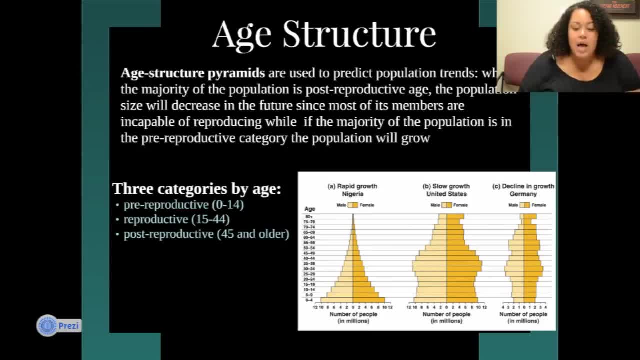 Age structure. The age structure pyramids are used to predict population trends. When the majority of the population is post-reproductive age, the population size will decrease in the future, since most of the members are capable of reproducing them, while the majority of the population is pre-productive category. 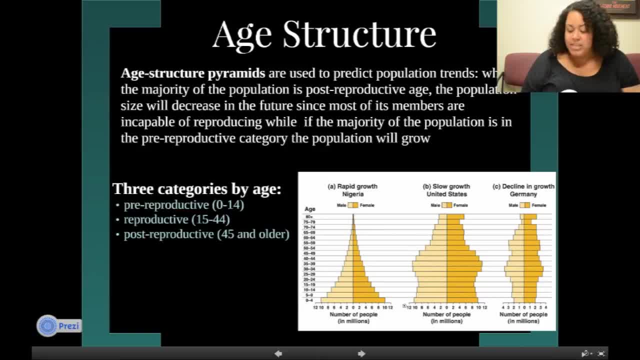 So everybody has something different. So, as you can see, in Niger, which has the largest people having babies right now, that's why most people are at a young age, While in the United States we have a steady growth rate but slow, because a lot of people are in the middle. 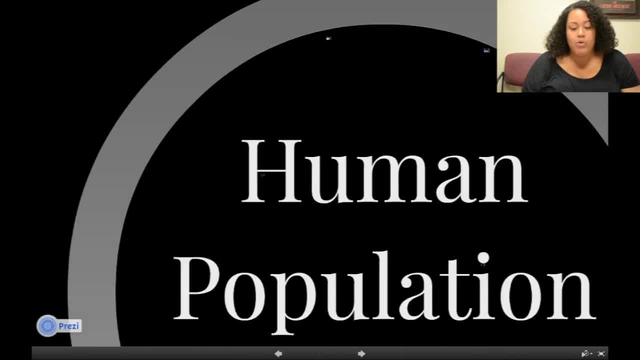 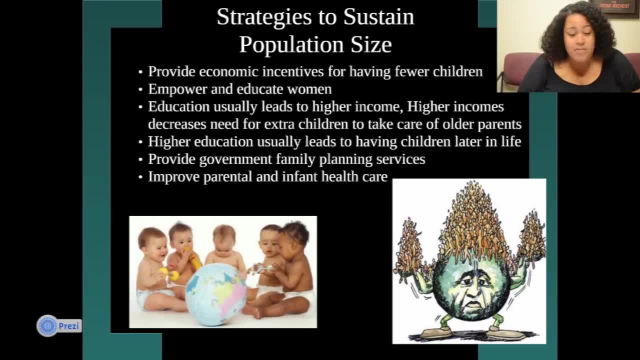 But in Germany most people are older because they have a declining growth rate. There are a lot of strategies. There are strategies to sustain population size. The reason why is to provide economic. some of the strategies are providing economic initiatives for having fewer children. 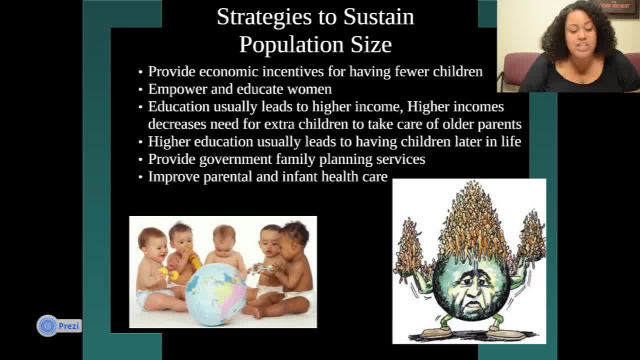 empower and educate women. education usually leads to higher income, and higher income decreases the need for actual children to take care of older parents. Higher education usually also leads to having fewer children later in life. Provide government family planning services and approve parental and infant health. 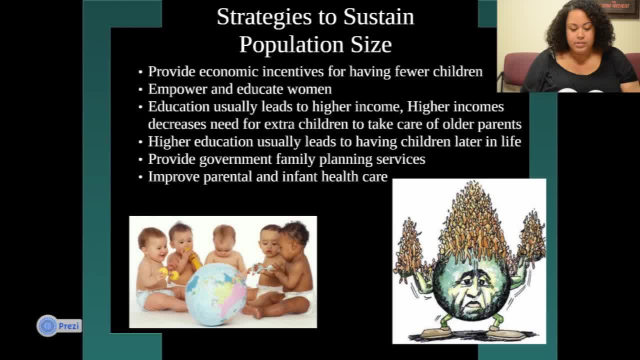 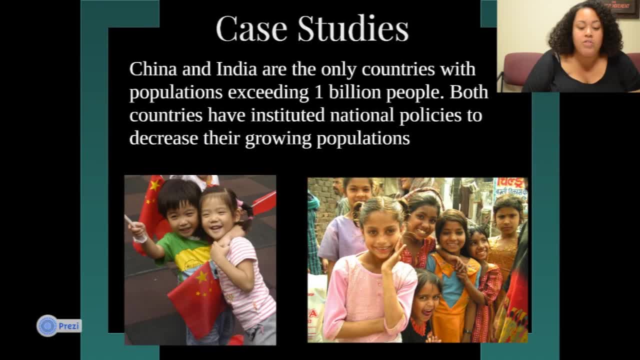 and provide health care. Here's some case studies about countries trying to decrease their population size. China and India are the only countries with populations exceeding one billion people. Both countries have instituted national policies to decrease their population growth. In China, they dramatically reduced their birth rate from 19 to 30 percent. 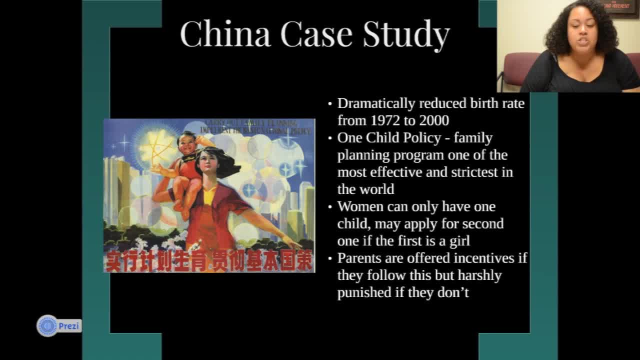 In China. they dramatically reduced their birth rate from 19 to 30 percent In 해서 in 2022 to 2000.. One of the biggest contributors to this was the One Child Policy. This was one of the most expected and stricted in the world. 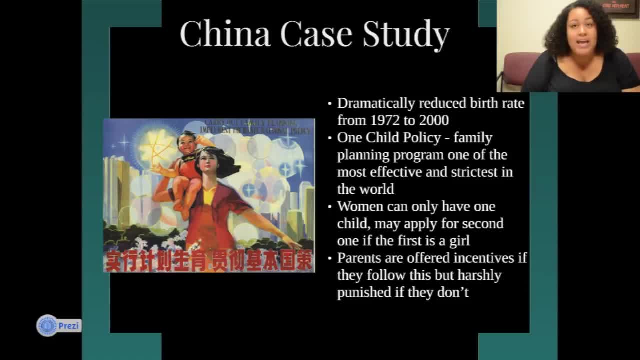 Laws and conditions allow people to be forced, and should be, sterilized if they have more than one child, but may apply for a second one if the first child is a girl. Parents are offered initiative if they follow follow this, but are harshly punished if they don't again. 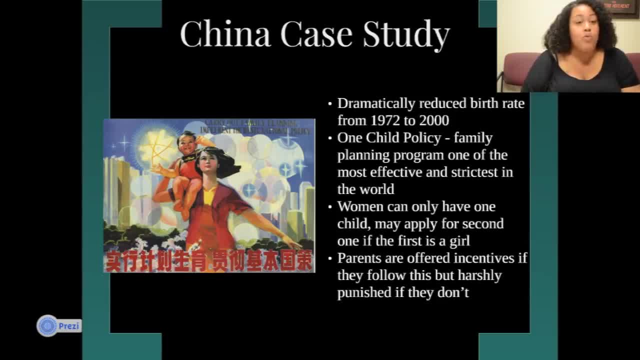 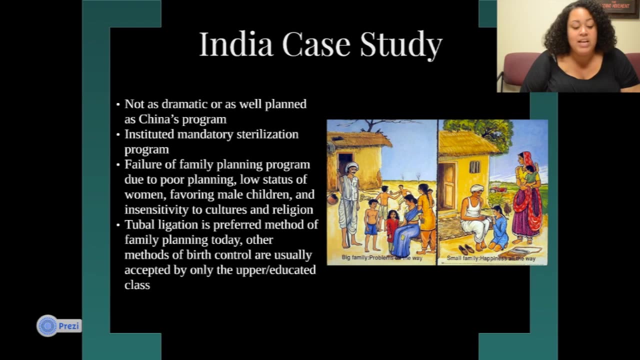 they can be harshly fined or served jail time for having more than one child. the India is not was definitely not as strict as China and not as well planned, but it instituted a mandatory sterilization program. the failure of the planning program was due to the poor planning, the low status of women and 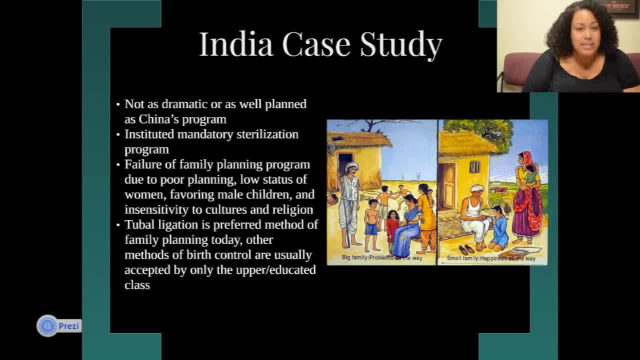 favoring male children- and insensitivity- insensitivity to the cultures and religions that India has. um. most people like to get their tube size the preferred method of family planning. today, that's usually for the upper and middle class, more educated and still trying to get more family planning. 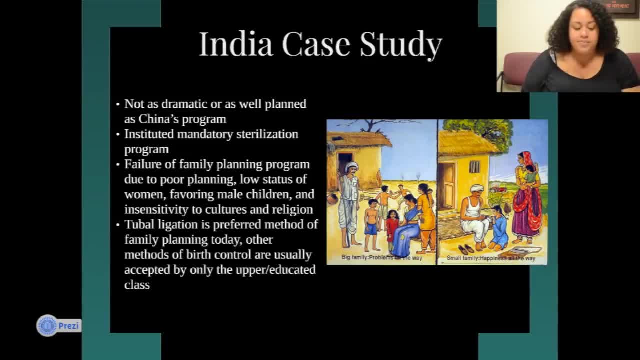 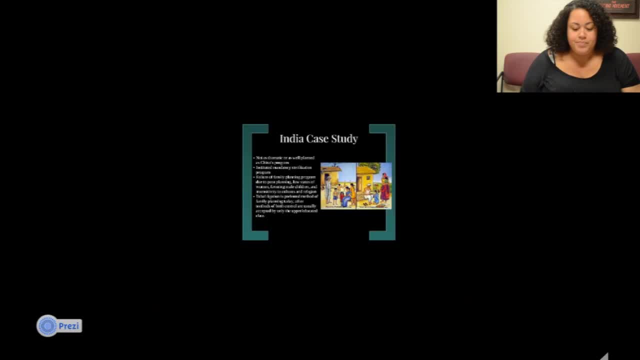 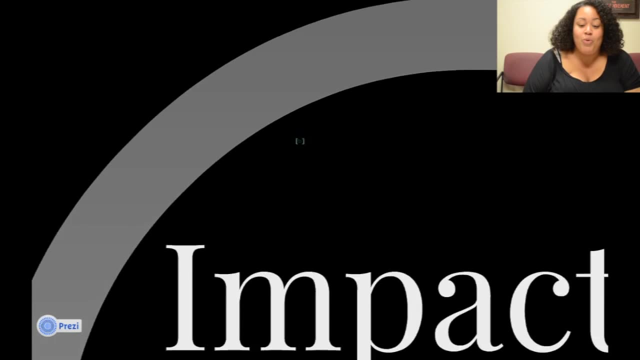 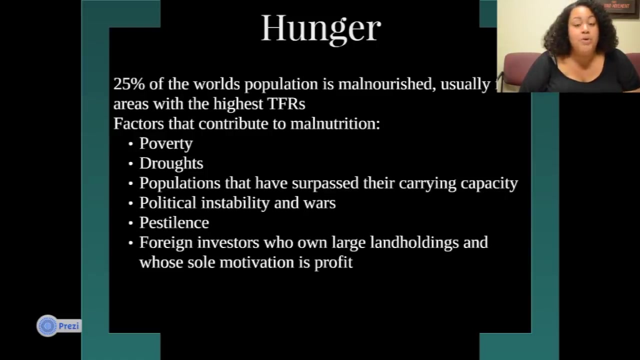 methods within the lower income communities. so impacts of population growth: hunger is one of the biggest impacts. 25 percent of the world's population right now is the malnourished and usually from areas with the highest tf r's. doctors that contribute to amout mutation, property, droughts, populations. 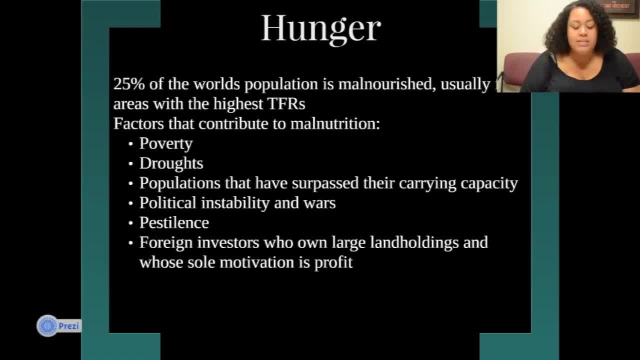 that have to pass to carry capacity. political estate. that's a ability. wars and wars, and foreign investors who own large land holdings and whose sole motivation is profit. As you can see, it's not because of a lack of food, it's because of political instability and social issues that people 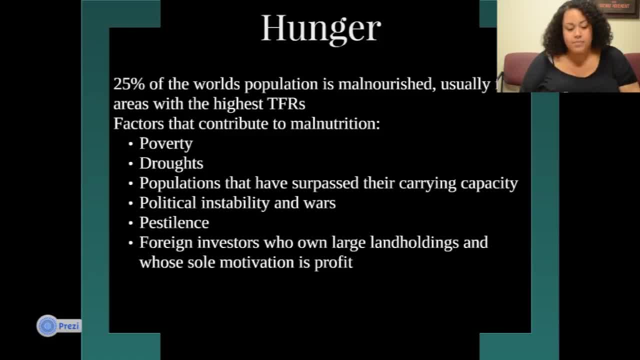 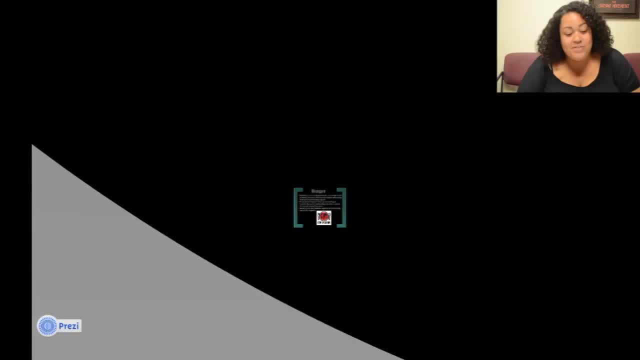 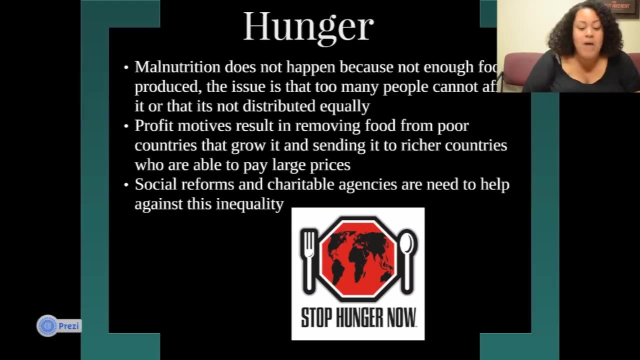 lose access to the food that is available. Malnutrition is again like I said. malnutrition does not happen because not enough food is produced. The issues: too many people cannot afford it or it's not distributed equally. Profit motives really result in removing food from poor communities. that 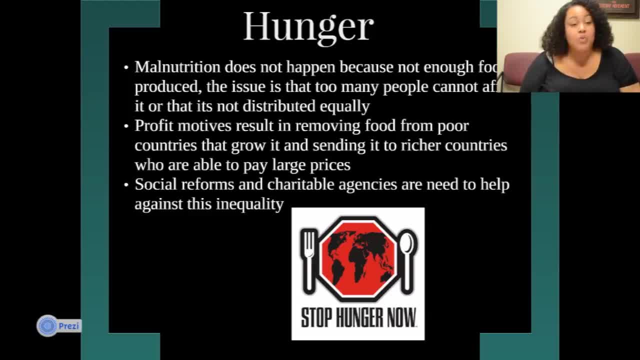 grow it and sending it to richer countries able to pay for large quantities of the food. For instance, a lot of our food, a lot of the fruit, fruits are from here that we get here are going to the Caribbean but those are being removed from the Caribbean people that want to access that food for us to. 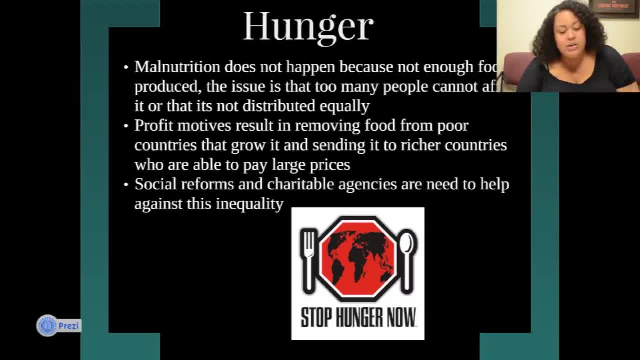 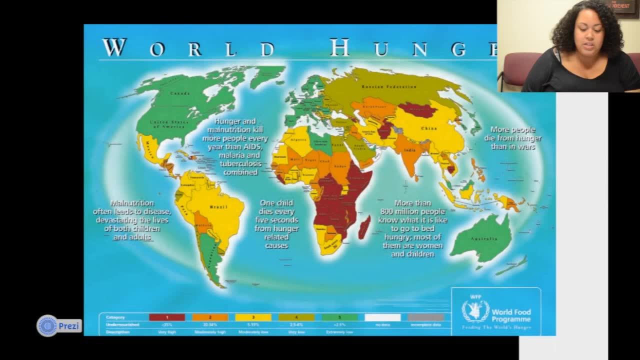 eat here and America. Social reforms and charity organizations are needed to help against this inequality. This map shows the world hunger around the world. so, as you can see the um, the more red it is, the more people are malnutrition there and the more green it. 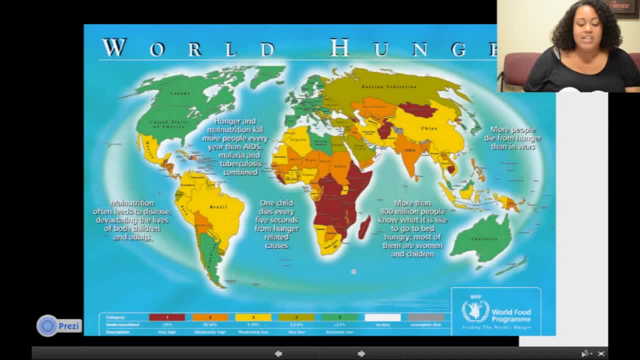 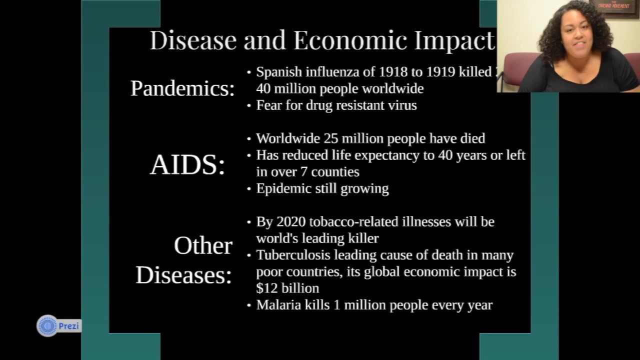 is. this is where less people are malnutrition. As you can see, it's mostly red Red in less developed countries and countries that have high are growing more rapidly than the more developed world. Disease and its economic impact. So pathogens, for instance. Pathogens are. 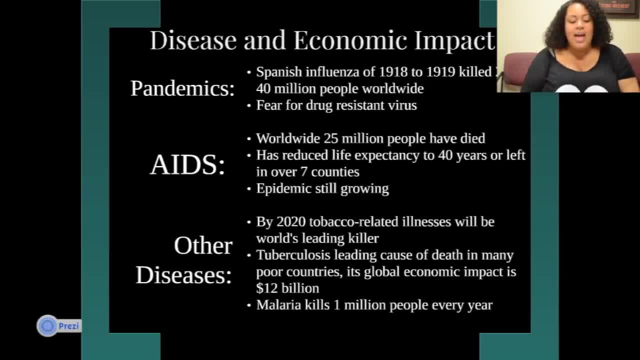 things like the flu and other things, and really it's fear for and it's really the fear of resistant viruses are bad. I mean pandemics, Like for pandemics- think about swine flu, like, way back in the day, AIDS, which is a worldwide issue. so far, 25 million people have died from it. 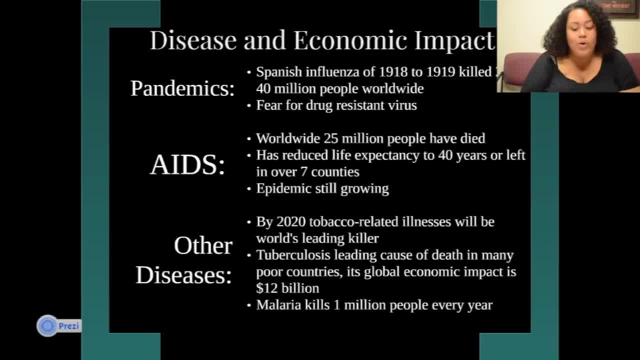 It's reduced the life expectancy to 40 years or and left or less in over like seven countries. The epidemic is still growing around communities around the world. There's other diseases. By 2020, tobacco related illnesses will be the world's leading killer. Tuberculosis is the leading cause of death in many poorer. 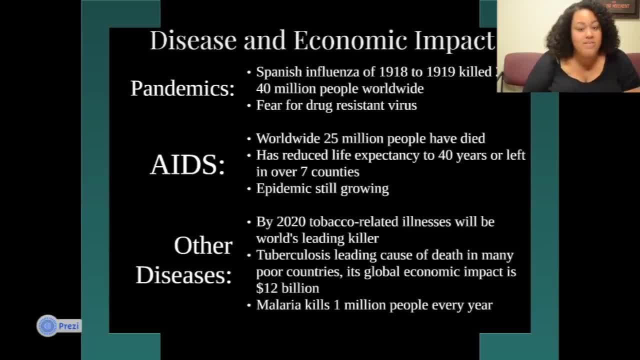 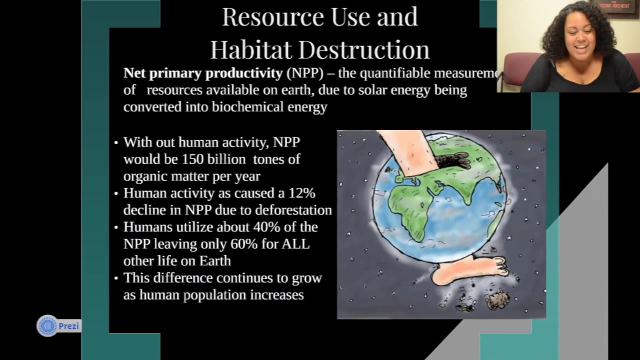 countries and its economic impact is 12 billion dollars. Malaria kills about 1 million people every year, which and there's also another disease that can be fixed by access to clean water. Next, we have the fact that there's a great deal of pollution and outrages on the planet. 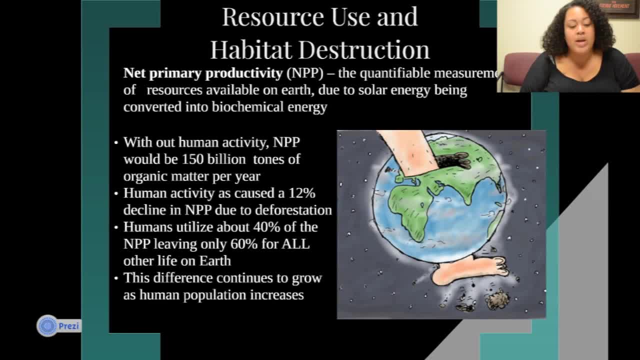 and evennin. So let's get on with it. Resource use and habitat destruction- and, believe me, habitats are being destructed. So net productivity- and pp is the quantifiable measurement of resources available on earth- You just store energy being converted into biochemical energy. What does that mean? That means that what resources that we have available to us and how we use them. So human activities have to be included or not included. Can that be a big deal? 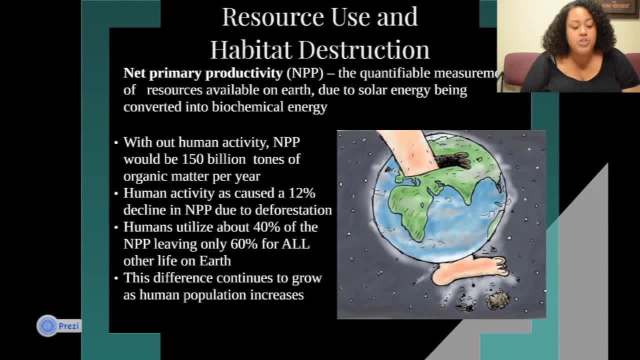 has caused a 12-degree decline in NPB due to deforestation and human-driven climate change. Humans utilize about 40% of the NPB, leaving only 60% for all other life on Earth. Humans don't make up that much of Earth's population. The fact that we take up the majority 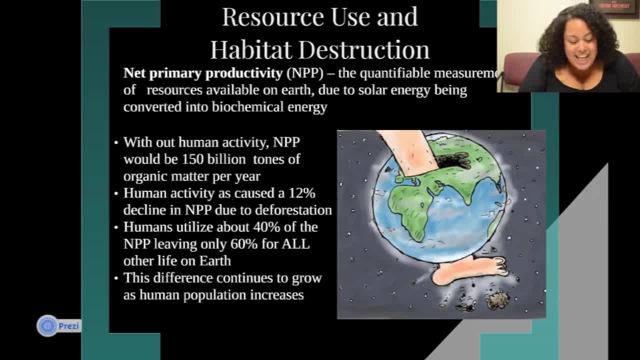 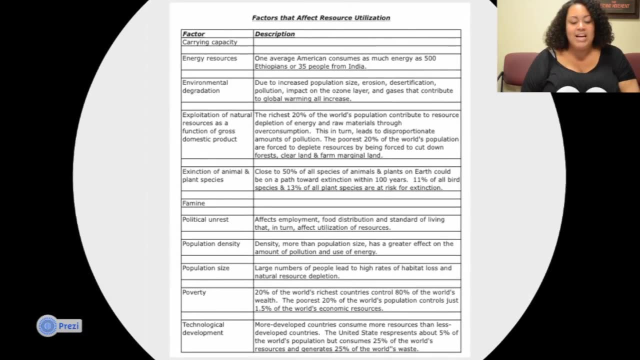 of it is a little bit of a problem. This difference continues to grow every day as a human's population increases. Here are some factors that affect resource utilization: The carrying capacity, energy resources, environmental degradation, exploitation of natural resources as a function. 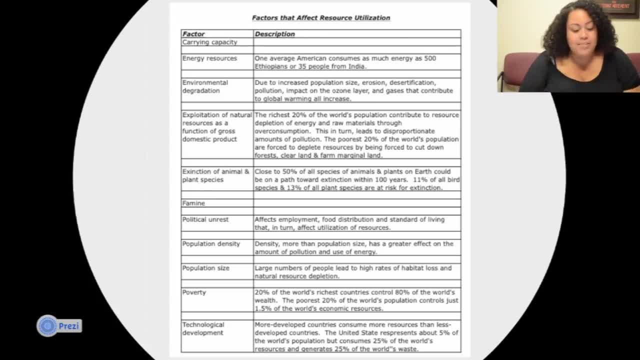 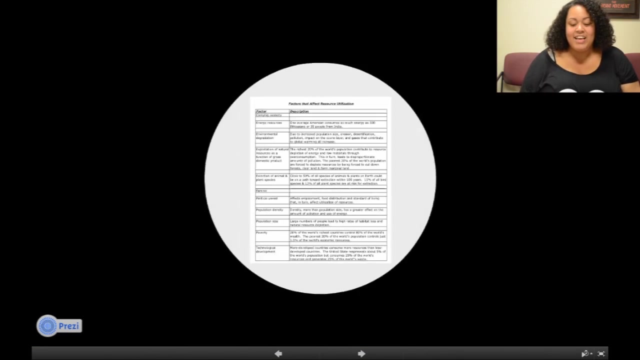 of gross domestic product, extinction of animals and plant species, famine, political unrest, population density, population size, poverty and technological development. Feel free to pause this video and read more about this graph. So that's it for population, you guys. Thanks for listening. This is the end, Good luck.